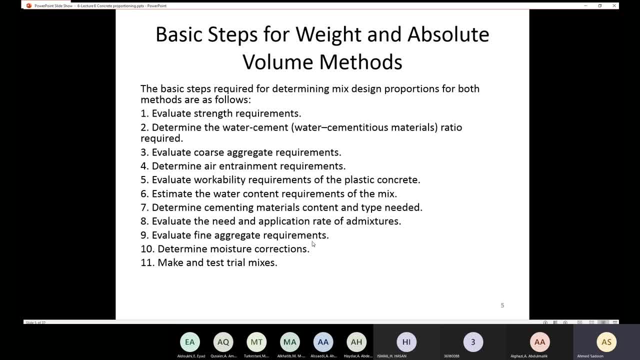 The proportions of the coarse aggregate, cement and the water should be such that receiving concrete has the following properties: Theuluð has the following properties: TheCómo you choose to verbatim grabbing a stream and then removing a bakalım is the one she's saying. 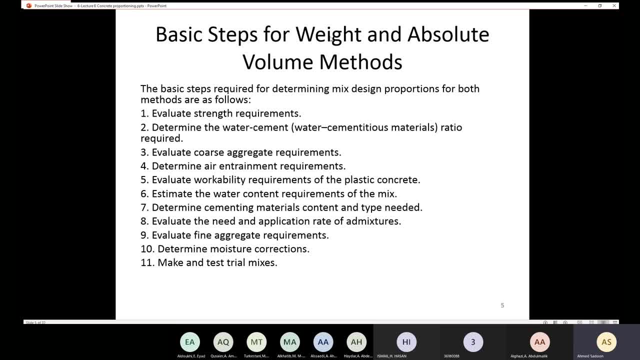 Both are true properties and the both are true solid properties. Some of what you should do is: What if the chance cost this for the motor to recover? Some of what you should do is: Todayных storage is Não é, não há não In. todayных storage actually is only foracağım obrig fleet or Chinese. 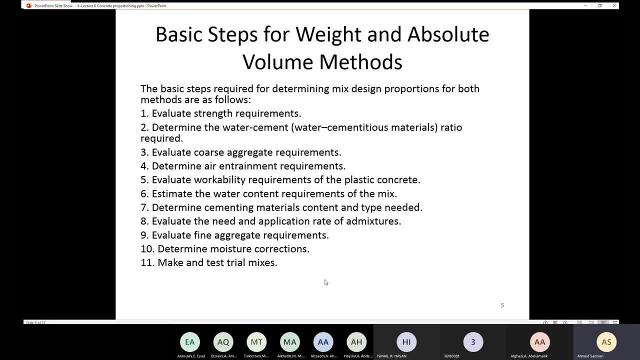 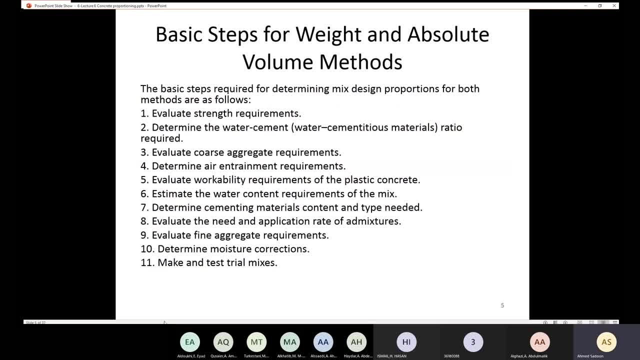 The good quality does not evenly in that one day. So do you have any questions up to that point? Do you have any questions up to that point? Okay, let's continue. I have we say that the first step is to evaluate the strength requirement. 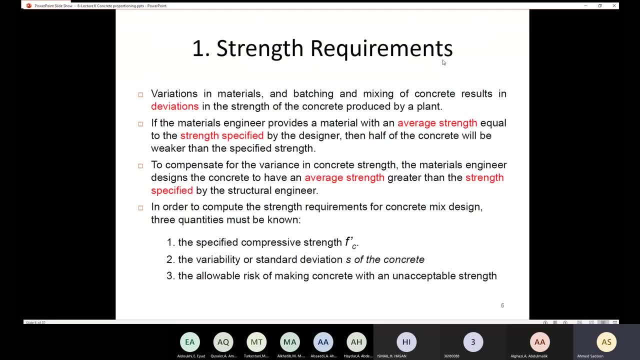 So now we are going to start the first step And we discuss the variation in the materials. We say that we have variation in the materials. So if you have sample for the same materials, Let's say you have three samples, like you have seen in the lab. 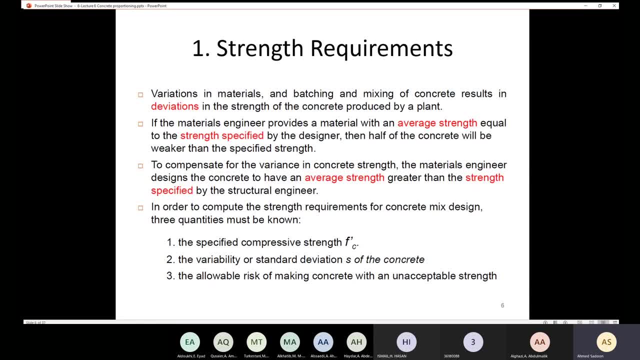 I'm not going to get exactly the same compressive strength for each sample. We are going to have variation And that is due to the nature Of the material. So variation in materials and the batching and the mixing of concrete Result in deviation in the strength of the concrete produced by a plant. 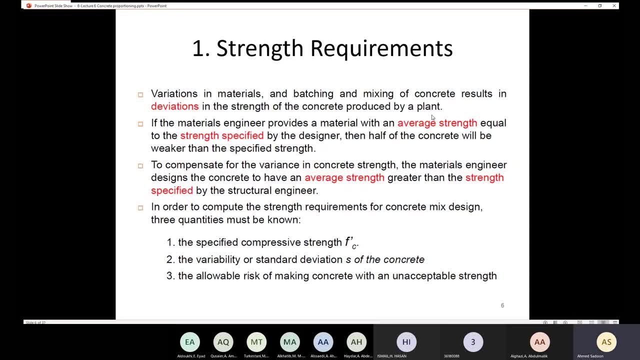 So the concrete that produced by the plant, I'm going to have variation. So if the materials engineer Provide a material with an average strength Equal to the strength of the material, So we are going to have variation. So if you have three samples- Sample 1, 2 and 3- 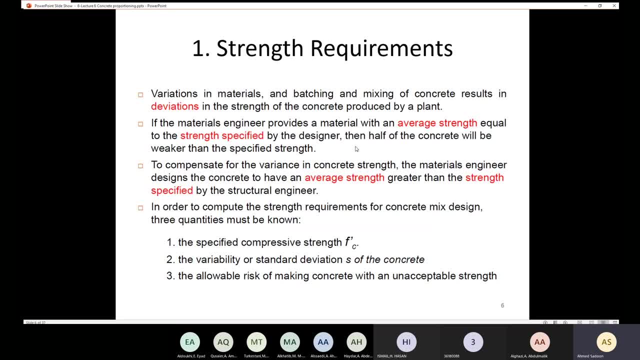 The strength for sample 1 is 15 MPa. The strength for sample 2 came out to be 20 MPa And the strength- the compressive strength- for the third sample Came out to be 25 MPa. Now, if you are going to get the average strength, 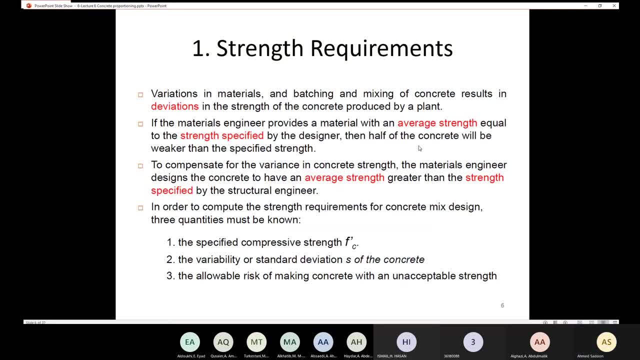 Of the material. The average strength is going to be 20 MPa. Now, if you are going as material engineer, If you are going to design the concrete With the average strength That it has been specified by the designer, Then the risk that the concrete is going to be lower than the average strength. 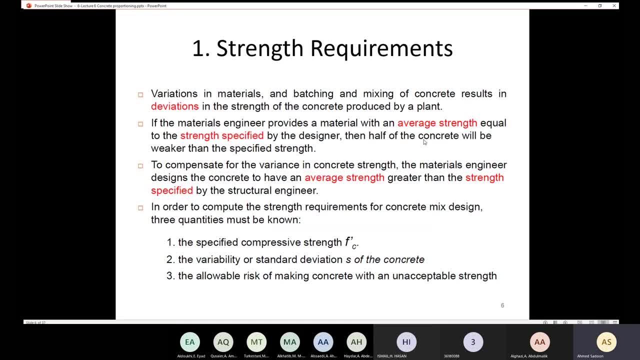 Is going to be 50%, Which means that half of the concrete Will be weaker than the specified strength, Because you Design based on the average strength. So I have a problem here And that problem is not acceptable. I'm not going to. design Depends on the average strength. 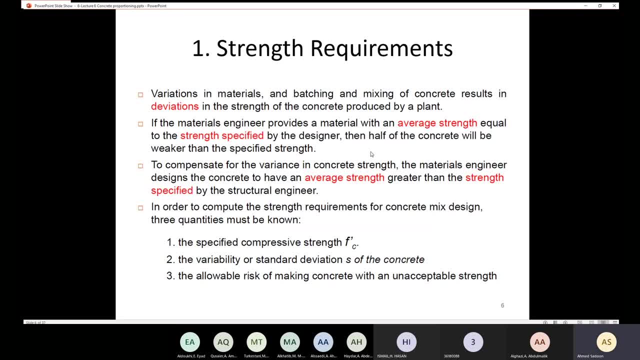 Specified by the designer, Because the risk is going to be 50%. So to compensate for the variance In the concrete strength, The material engineer Designed the concrete to have an average strength Greater than the strength Specified by the structural strength. So the structural engineer, 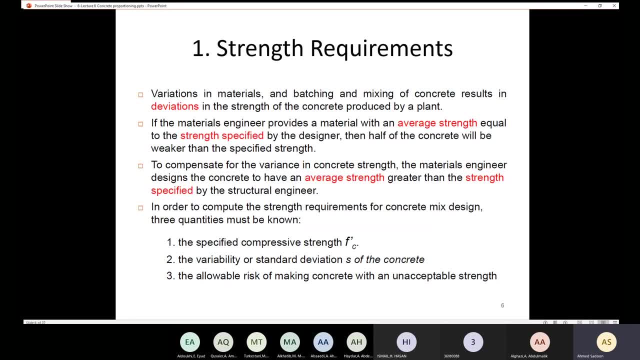 Is going to give you The average strength. He said that I need average strength, For example, 20 MPa, But, as material engineer, If I'm going to design Based on what the Structural engineer, Or the designer, again Based on what he has said, That is going to put me on a risk of 50%. 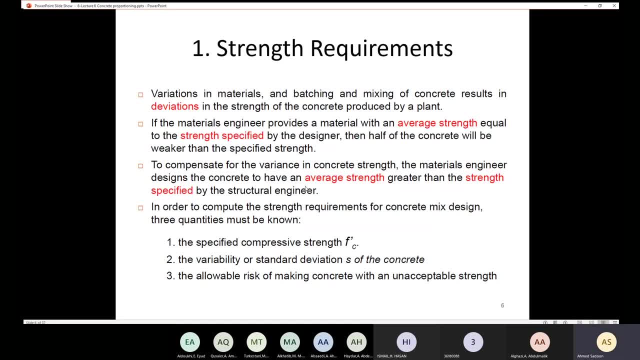 So the solution is: I need to design More, More, More, More Than the average strength. So in this case, We are going to See the risk. I need to know the allowable risk. Normally, The allowable risk Is going to be 10%. The allowable risk Should be 10%. 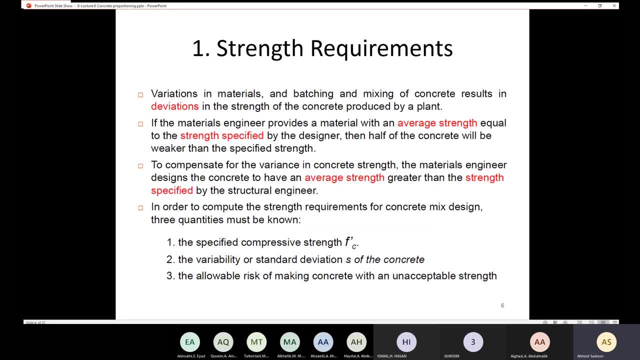 So, in order To have a concrete With allowable risk 10%, I need to use a statistical model. I need to use a statistical model. So, in order to use A statistical model, We are going to assume normal distribution. And in order to assume normal distribution, 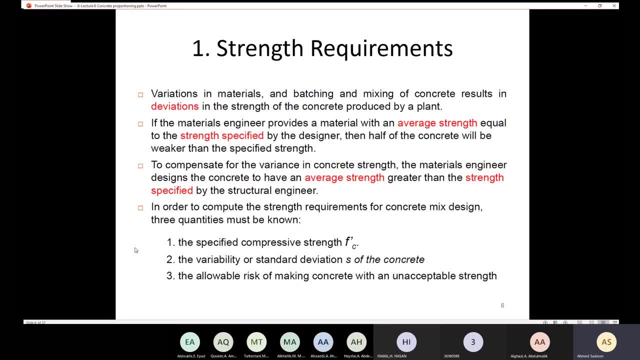 I have to know many information, Or three information. First information: I need to know the specified compressive strength And also I need to know the variability And the standard deviation. S I need to know the standard deviation And also I need to know the allowable risk Of making concrete. 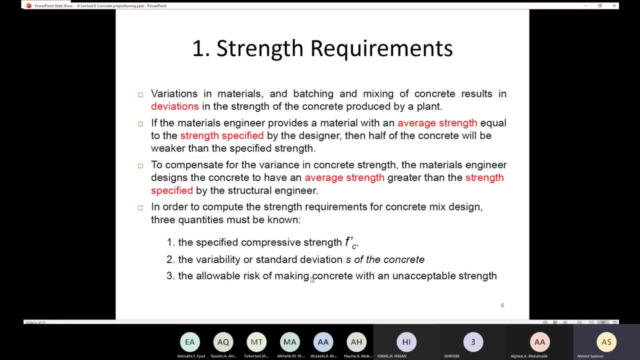 With unacceptable strength. So I need to know this And this And this If I'm going to know the allowable risk. I need to know the value of Z. So those who took a statistical method course, They know They are familiar with the value of Z. You have a certain table. 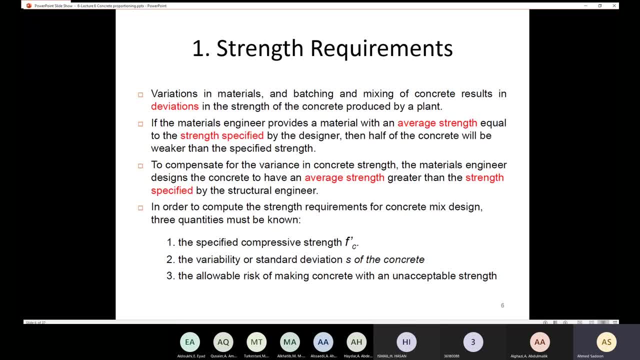 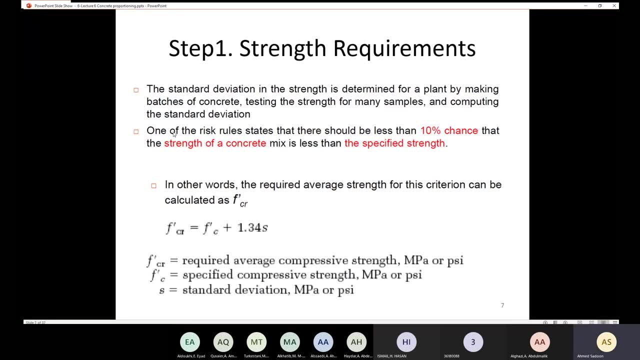 If you know the value, If you know the risk, The probability of the risk, Then you will be able to know the value of Z. Then We are going to assume that The risk should not be less than 10%. So the risk should not be less than 10%. 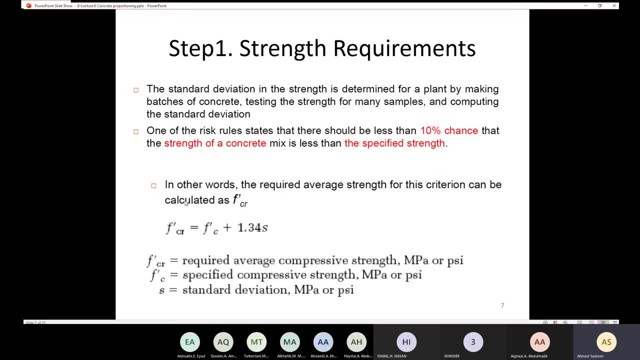 And we are going to use A statistical model, This model here, Which means that The required average compressive strength, Fcr- This one is the strength as material engineer I'm going to design based on this value. So the Fc is the value of Z, The value specified by the designer. 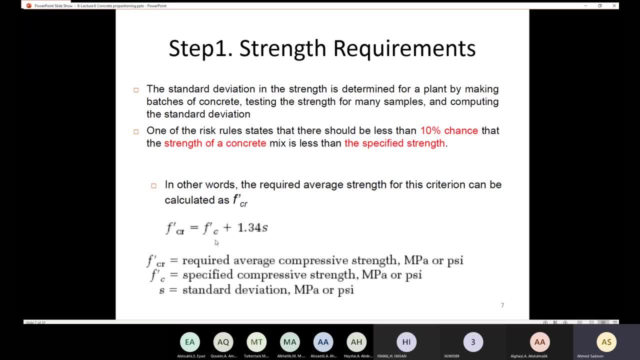 Or the structural engineer. I'm not going to design based on that value. I need to add: I need to design more than that value, But with a risk Should be less than 10%. Like I said, This formula here depends, Or we borrowed this formula From the statistical method. 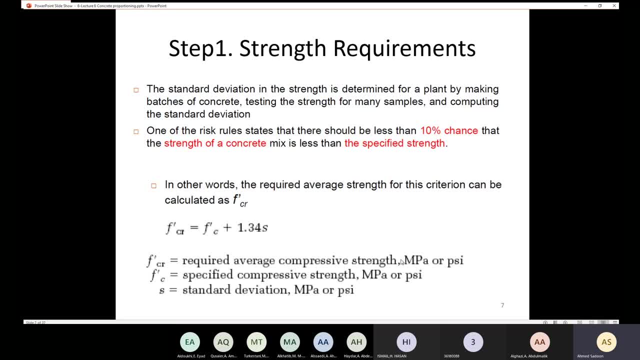 So now, Fcr represents the required average compressive strength By megapascal or pci. Fc is the specified compressive strength. So this one- It has been determined By the designer- And this one Is going to be the Compressive strength The material engineer is going to design with it. 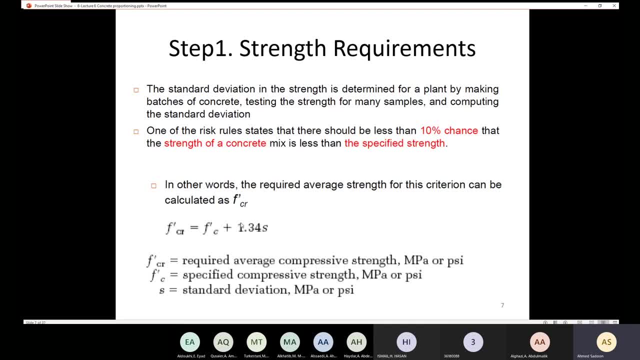 So I have Fcr and I have C Plus 1.34. 1.34 represents the value of Z, The value of Z depends on the risk And S represents the standard deviation. So now I'm going To sum up all of this. I'm going to design. 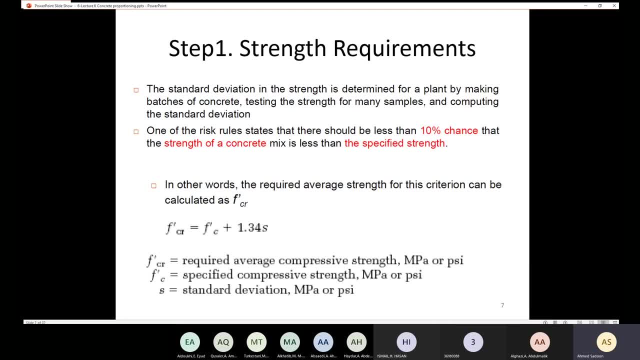 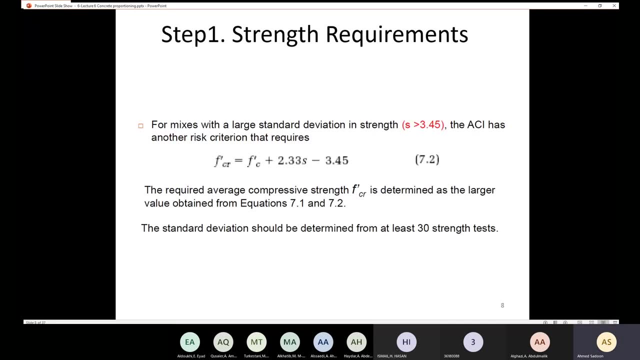 With compressive strength More than the average compressive strength Determined by the structural engineer. In order to do that, I'm going to use this formula. Okay, And this formula, it has conditions. The value of S Should be less than 3.45 If the value of Z 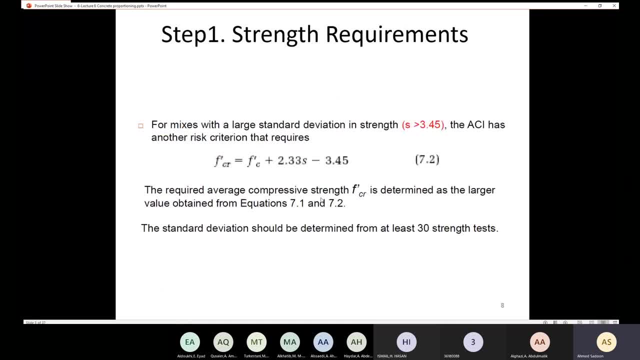 Which is the standard deviation, Is more than Is more than 3.45, Then I'm going to use another formula Borrowed from the statistical method, Which is this formula: So, if the value of S- The standard deviation- is more than 3.45, I'm not going to use this formula. 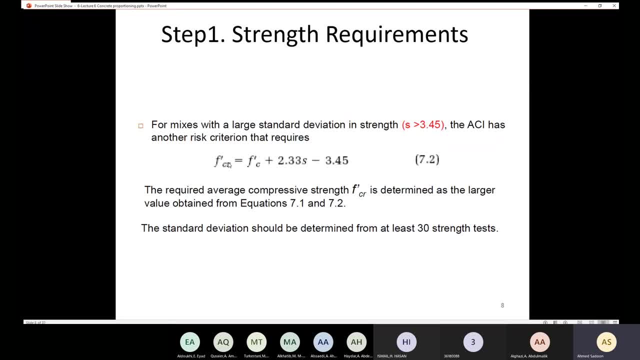 I'm going to use another formula, Which is here The Fcr. The compressive strength Specified by the material engineer Equal the compressive strength Specified by the structural engineer Plus 2.33. S is the standard deviation Minus 3.45. So if the standard deviation 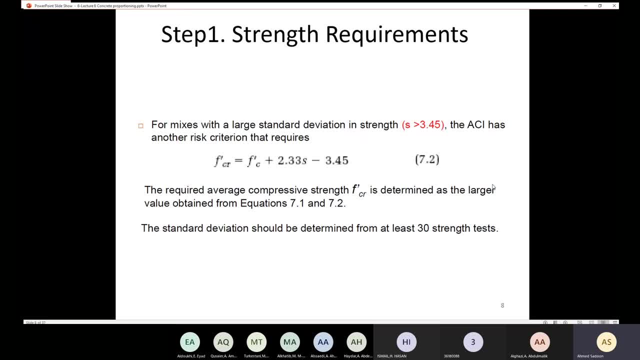 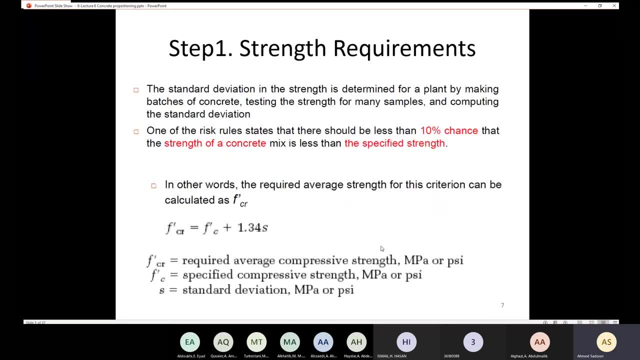 More than 3.45, Then I'm going to use this formula here. If you are confused about Which formula should I use, Should I use formula one or formula two? In that case, use both formulas: Substitute in the first formula And in the second formula. 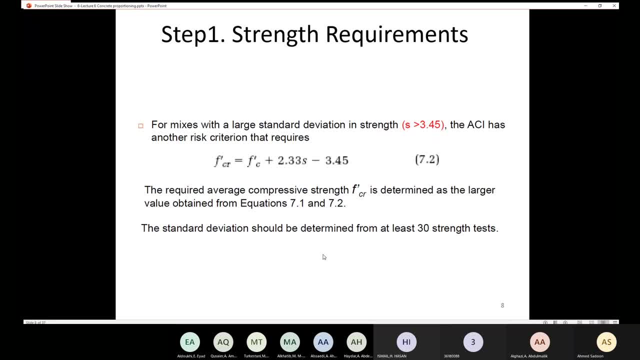 Then use the larger result, So this formula Will yield a result, And this formula also will yield a result. Use the larger value, So there required Every compressive strength, Fcr is determined as the larger value obtained from this formula. Okay, Let's go for a system. 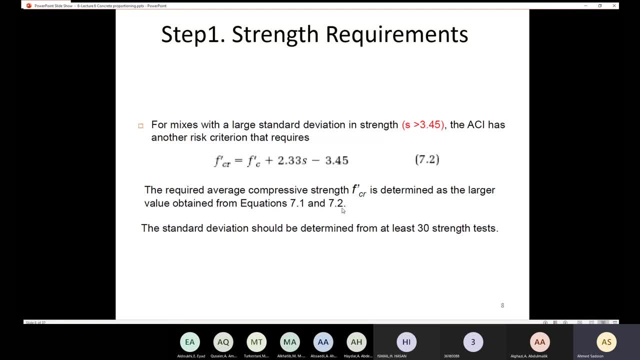 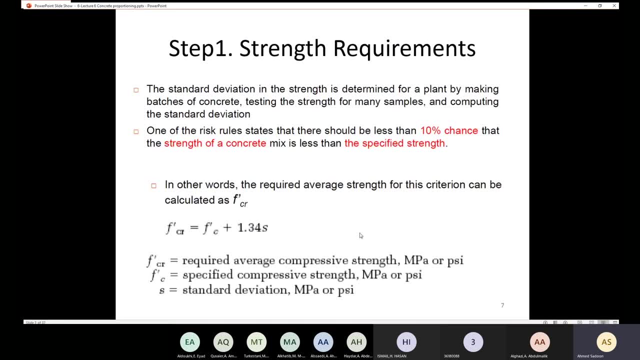 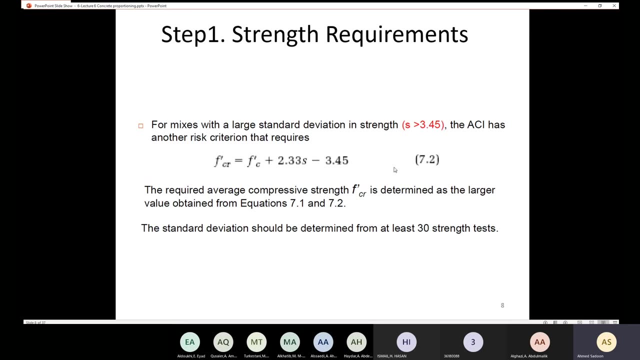 from equations 7.1 and 7.2. so, if you are confused, use the this formula. this formula is 7.1 and this formula, which is 7.2, and the formula that is going to give you the larger value. you are going to use that larger value and in order to 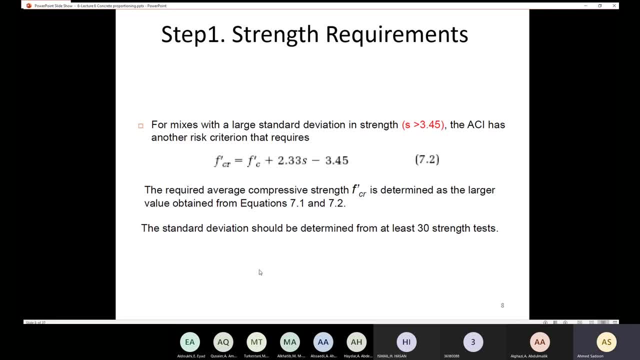 use these two formulas. you have condition for that. the standard deviation should be determined for from at least 30 strings tests. so I have condition for those formula, the standard deviation. of course you are going to determine the standard deviation based on the number of these samples from the concrete plant. 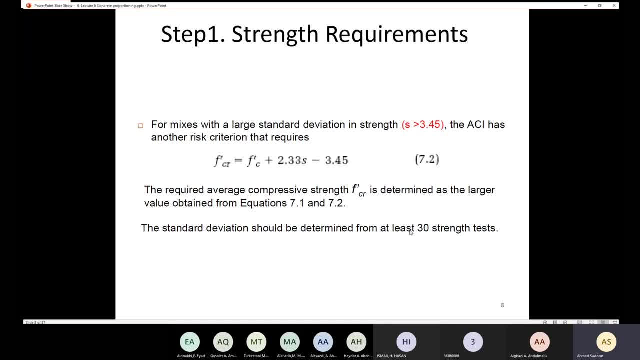 and the number of sample should be at least 30 samples. otherwise I have other options for that. I need to correct the value of the standard deviation. so if the numbers of the of the specimen is more than 30 samples, then I need to apply a correction factor for the standard deviation. let's see the 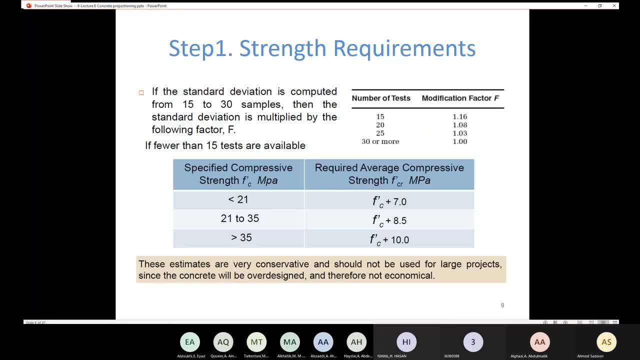 standard, the correction factor, if the standard deviation is computed from 15 to 30 samples. so if your samples between 15 and 30, then a standard deviation is multiplied by the following factor correcting factor F. of course, if the your sample is more than 30, you don't need that factor which. 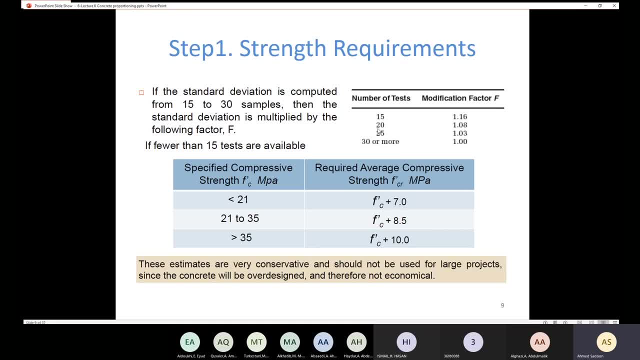 means that the factor is one. if your sample is 25, then you need to multiply the standard deviation by 1.03. if your sample is 20, then you are going to apply 1.08. if your sample is 15, then you are going to apply 1.16. as. 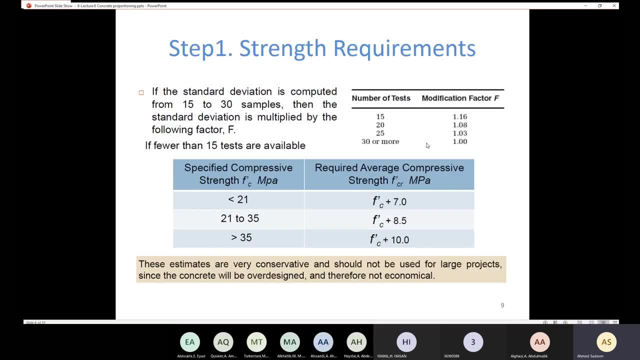 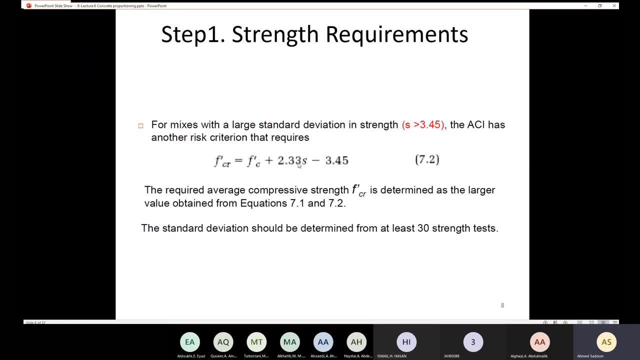 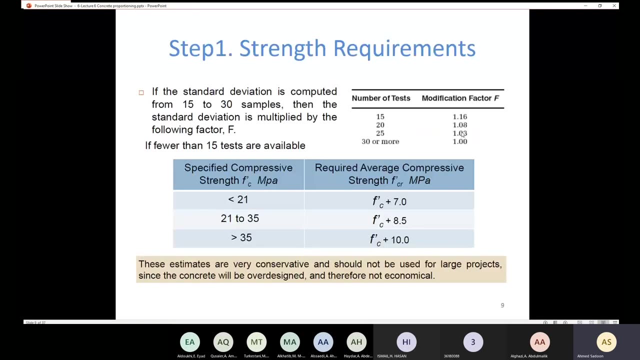 factor. so you are going to use this formula, but the value of s should be multiplied by the factor. for example, if your sample is 25 sample, then the value of s should be multiplied by 1.03. so now what if the your sample is fewer than 15 samples or 15 tests? in that case, i'm not going 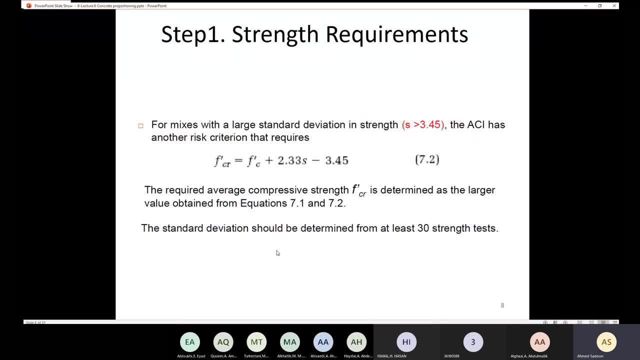 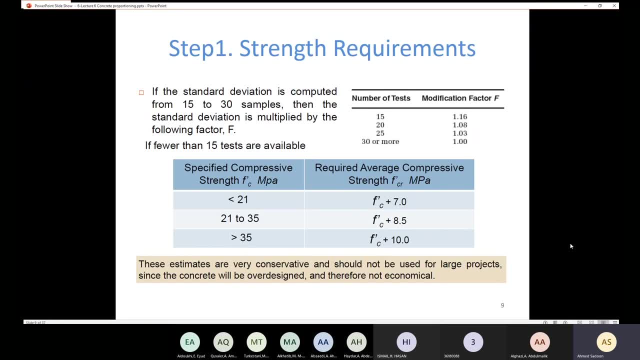 to use this formula at all. i'm going to use different formulas: either this formula or that formula or that formula. you are going to use this formula if the specified compressive strings is less than 21. you are going to use this formula here if your specified compressive 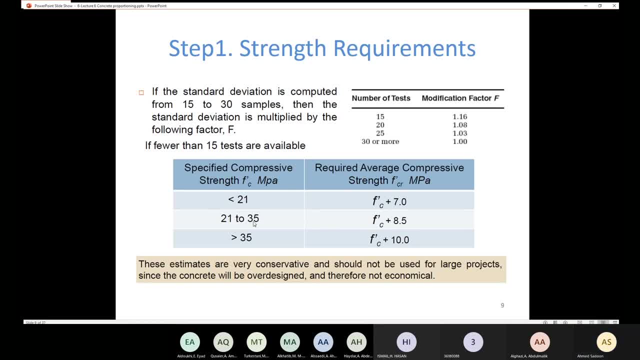 strings is between 21 to 35, you are going to use this formula here if your specified compressive strings is less than 21. you are going to use this formula here if your specified compressive strings is more than 35. so, to summarize this: if your samples is more than 30, 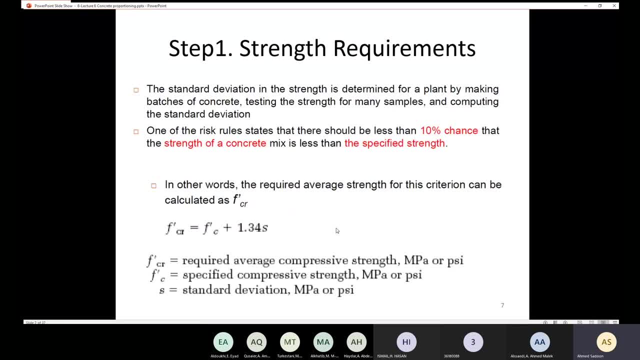 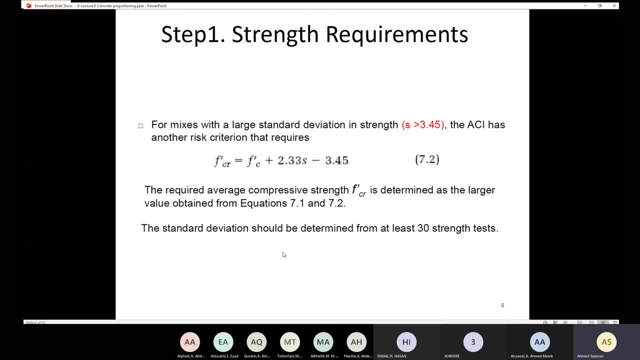 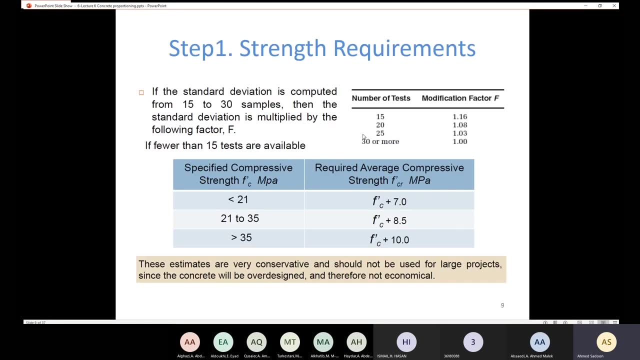 samples. in that case, i'm going to use this formula and that formula, and then i'm going to use the larger value if your samples between 15 and 30. if your samples between 15 and 30, then i'm going to apply a modification factor for the sample and i'm going to apply a modification factor for the. 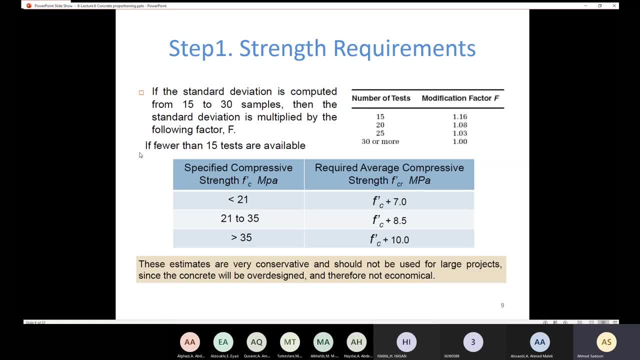 value of the standard deviation if your samples is less than 15 tests. in that case i'm going to use new formulas. either this formula or that formula or that formula depends on the specified compressive. to make the picture clear for you, let's see this example. 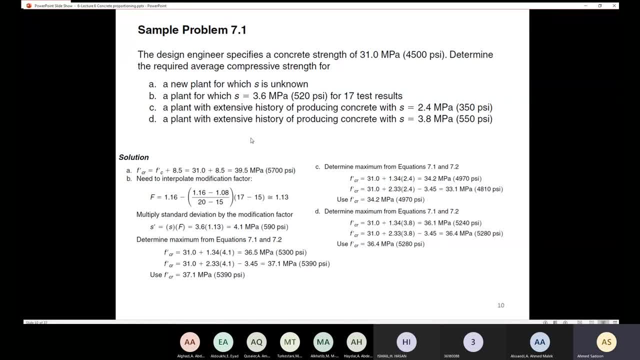 this example will help you to understand what i have mentioned in the previous slides in this. in this example, the design engineer specified a concrete strings of 21 mega pascal. this value has been specified by the design engineer. then it says that determine the required average strength for case one, case a, case b, case c, case d. so we need to know the compressive strings. 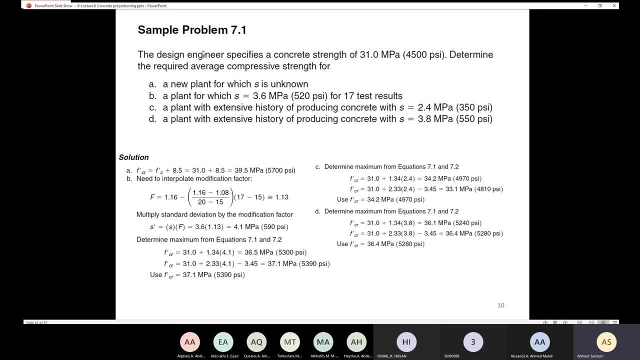 for the material engineer. so the value here for the designer engineer? we know that for the material engineer we need to use a value more than this value. for case number one, he said that your plant is a new plant for which s is unknown. so now you don't know the value. 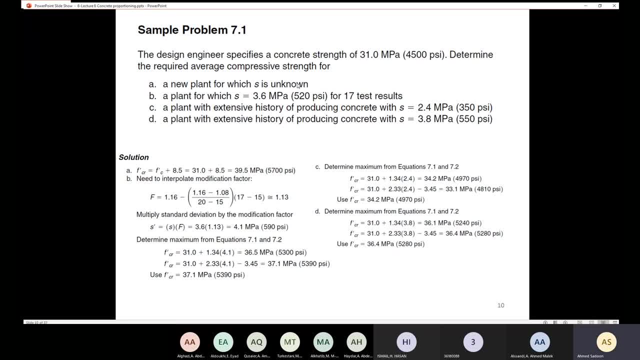 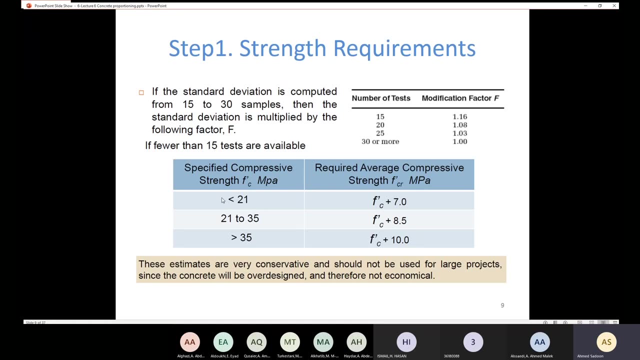 of s, the plant is a new plant. if your plant is new plant, that mean you don't have sample at all. you don't have any sample. so in this case i'm gonna say that the number of sample is less than 15 tests. so in this case i'm going to use this or this or this formula depends on the specified. 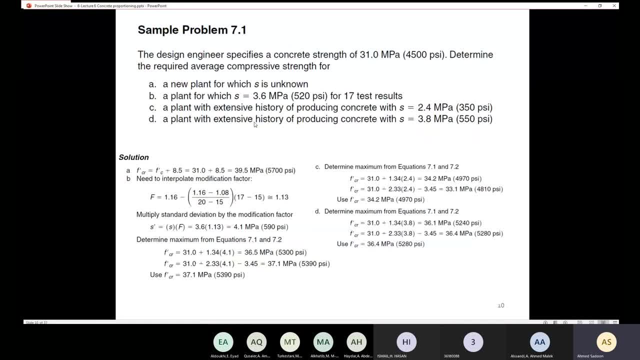 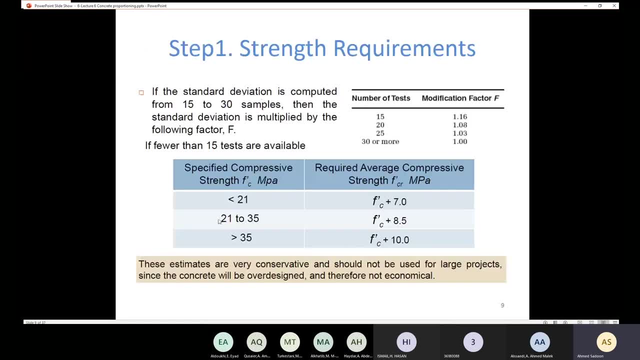 compressive string. so let's see what is the value of the specified compressive string. the specified of compressive strings is 31, so here 31. 31 is between 21 and 35, so in this case i'm going to use this formula here. so now the value of fcr is going to equal the value of fc plus. 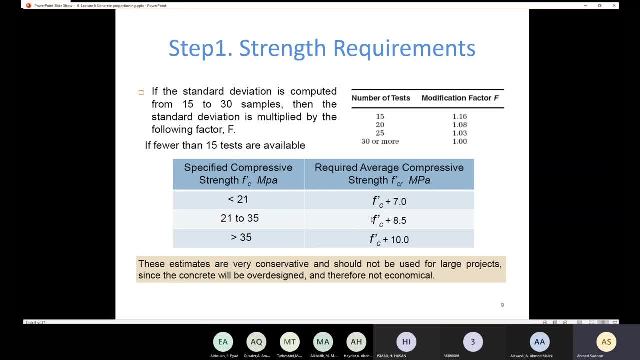 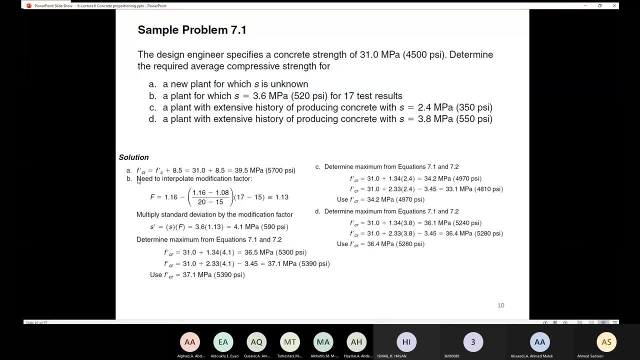 8.5, the value of fc is 31. so 31 plus 8.5 is going to give you the value of fcr. so for case a, the value of fcr is going to equal fc plus 8.5. the value of fc is here. 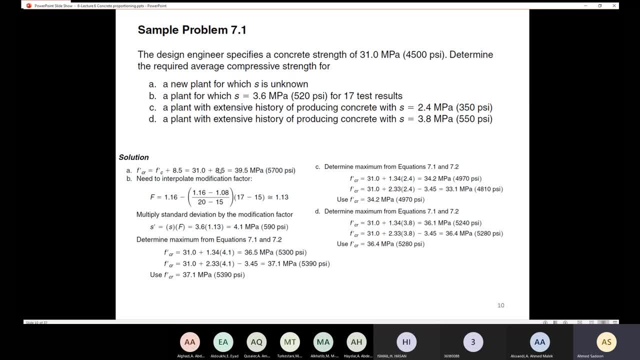 31. so 31 plus 8.5 came out to be 39.5 megapascal. so now that the, the, the material engineer, is going to design with this value, now i have case b. in case b, a plant for which the value of s now we. 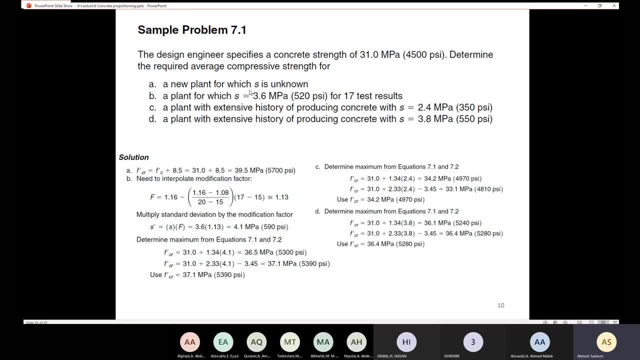 know the value of the standard deviation. uh came out to be 3.6 megapascal. for how many samples? i have 17 test results, so i have 17 sample. so, in this case, what should i do? so in this case, since i'm going to get back here, 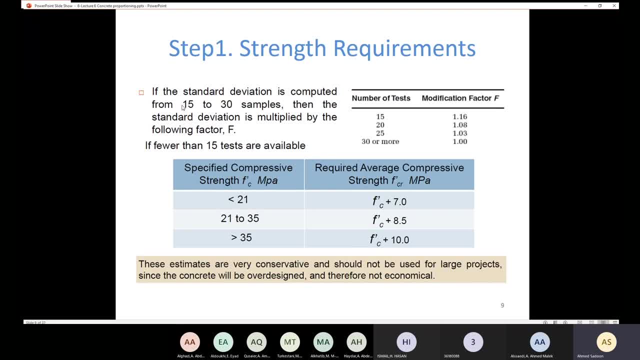 the number of sample is 17, which means that the number of sample is between 15 and 30, and the number of sample is 7- 17, so 17 is going to be between 15 and 20.. in this case, i'm going to use 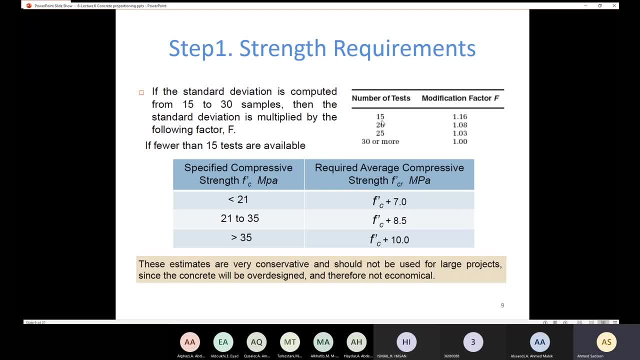 interpolation. in that case, i'm going to put 17 and the value of this is going to be x. i'm going to tables and then i'll be able to determine the value of x. we have done this in the lab so many times, so i think most of you familiar with the interpolation. so, because the value of 17 is, 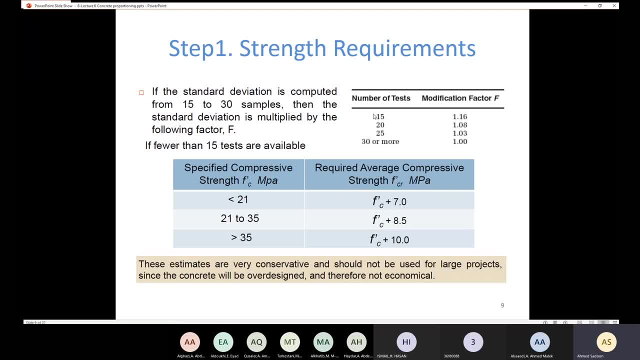 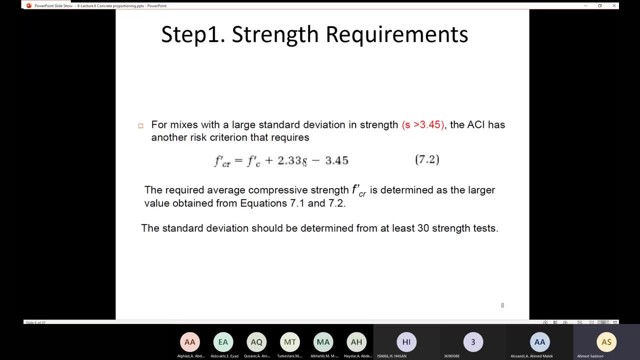 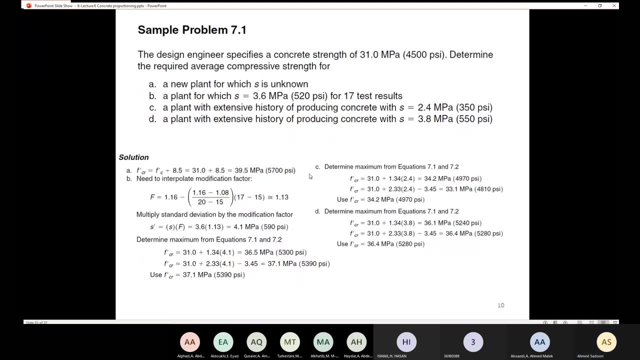 not listed in the table. i need to make interpolation. so i'm going to correct the value of s for this formula and for that formula. so the value of s should be multiplied by the modification factor. so this is the value of the modification factor. we say that we need to interpolate because the value of 17 is not listed in the table. 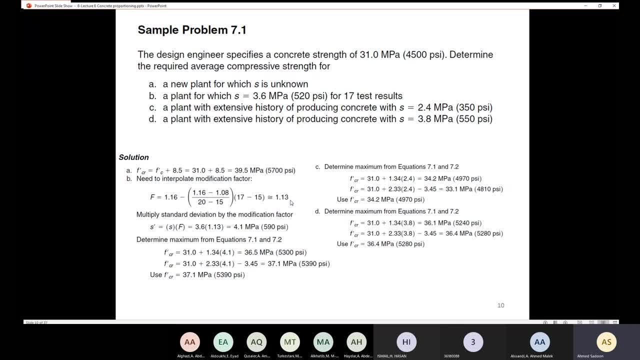 the modification factor came out to be 1.13. so the value of s, which is 3.6, should be multiplied by 1.13. the value of s come out to be 4.1, mega pascal, then i'm going to use the first formula, this. 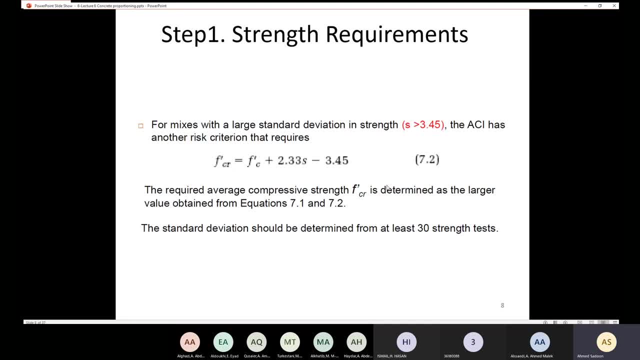 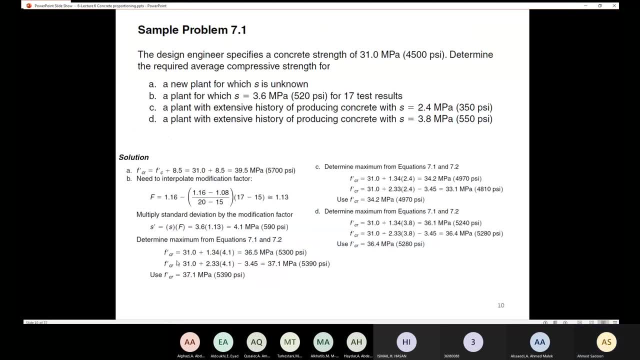 formula and the second formula and i'm going to get the larger value. so here i'm going to use the first formula and i'm going to use the second formula, but i'm going to use the modified standard deviation. and now, which one is bigger? the second formula is is the bigger formula, so i'm going to 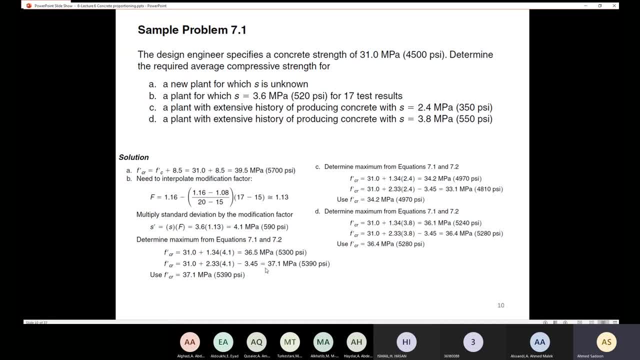 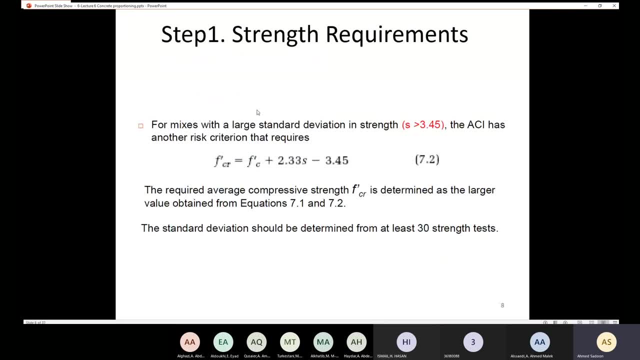 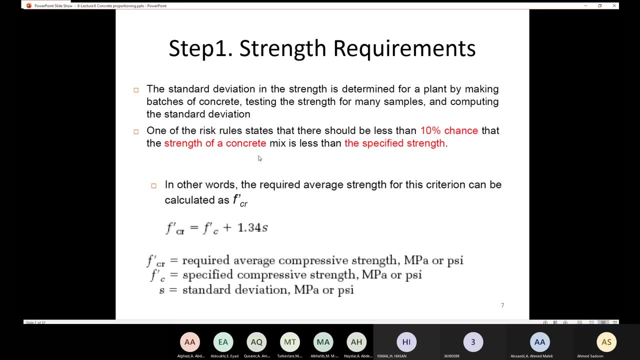 use this value here. or, if you are clever, you are going to say that, since the value of 3.6, this value is more than 3.45, so this formula should give me the larger value. okay, so, if you are, if you are not sure, you are going to use the first formula and the second. 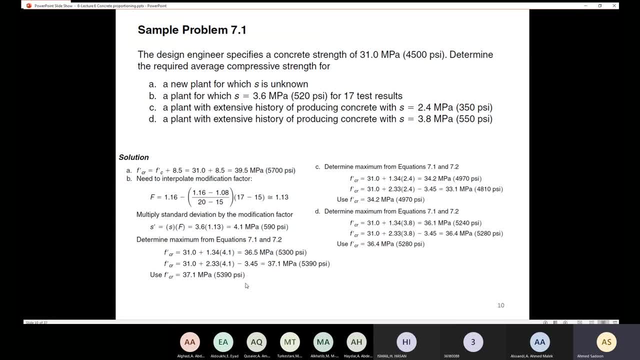 formula and you are going to use the larger value. similarly here, in plant c they say that the plant with extensive history, expensive history. that means the plant produced many samples. the samples is going to be more than 30 samples and the value of s came out to be 2.4. so in this case i'm going 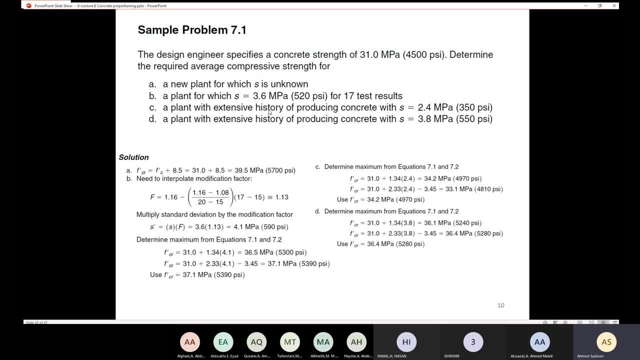 to. i'm going to say that, since i have extensive history, the number of samples is going to be more than 30 samples. i'm going to use the first formula and the second formula and i'm going to use the larger value. of course. the value of s here, 2.4, is less than 3.45, which means that the first formula is going. 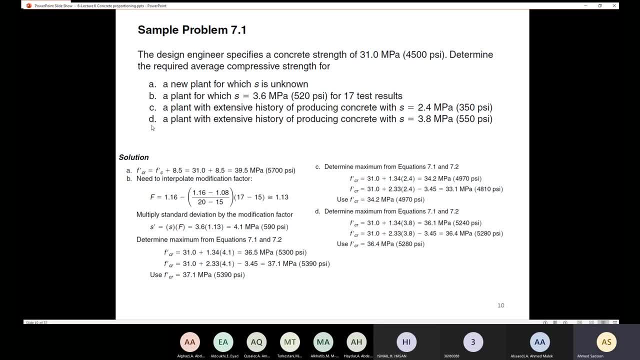 to give me the larger value. finally, number d, the plant with expensive history of producing concrete, which means that extensive history, the number of samples is going to be more than 30, which means that i'm going to use the first formula and the second formula and then i'm going to use a larger value. but again, if you are clever, you know that the value 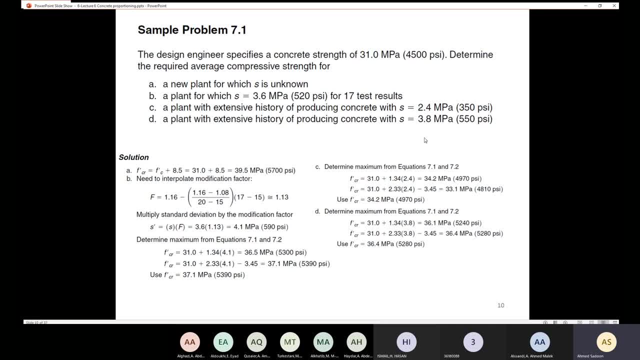 of s is 3.8, which is more than 3.45, which means that the second formula is going to give me the larger value. i'm going to stop here at that point. i'm going to give you the floor for questions. 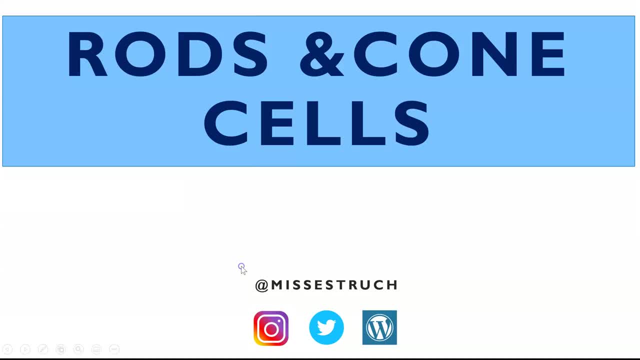 Hello and welcome to learn A-level biology for free with Miss Estrick. In this video I'm going to go through rods and cone cells as photoreceptors. So click here if you haven't subscribed already, to make sure you don't miss out on any of the videos. So just a little bit about receptors. 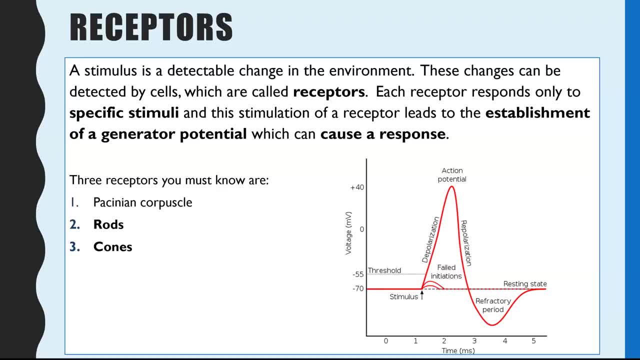 These are the cells which detect a change in your environment, and each receptor responds to a specific stimulus And once they respond, if the stimulus is big enough- so if the change in the environment was big enough- it will lead to an action potential. And you can watch here. 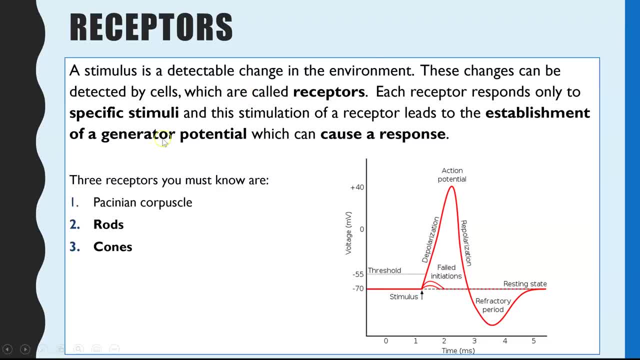 my video on action potentials to find out more. Now in this video I'm just going to be going through rods and cones. I already have a previous video on the receptor, Bicinium corpus school, which again I'll link here so you can have a look. So I'll be looking at the